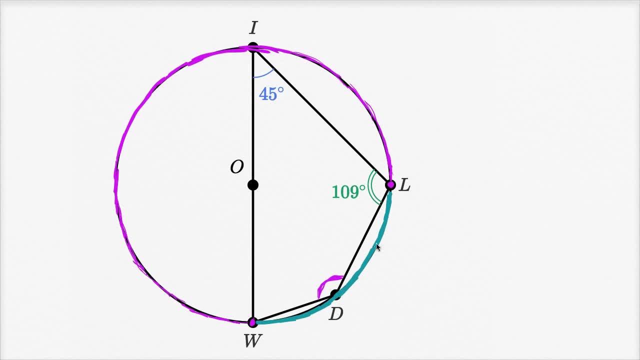 then this over here is a 90 degree arc. The measure of this arc is 90 degrees. The measure of arc, I guess you could say this is the measure of arc. let me write it this way- The measure of arc WL. 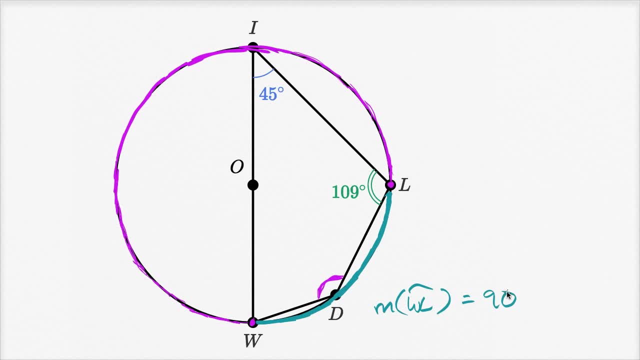 is equal to 90 degrees. It's twice that the inscribed angle that intercepts it. Now, why is that helpful? Well, if you go all the way around the circle, you're 360 degrees. So this purple arc that we cared about. 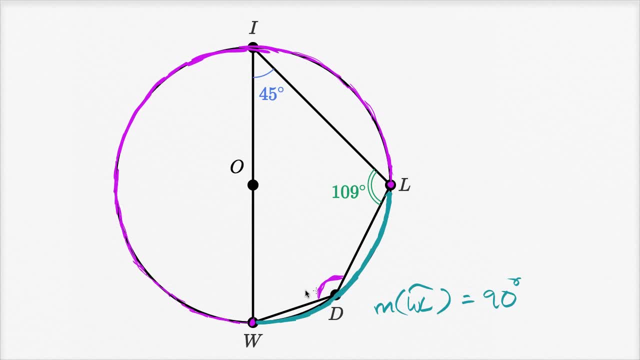 that we said, hey, if we could figure out the measure of that, we're gonna be able to figure out the measure of angle D. that plus arc WL, they are going to add up to 360 degrees. Let me write that down. 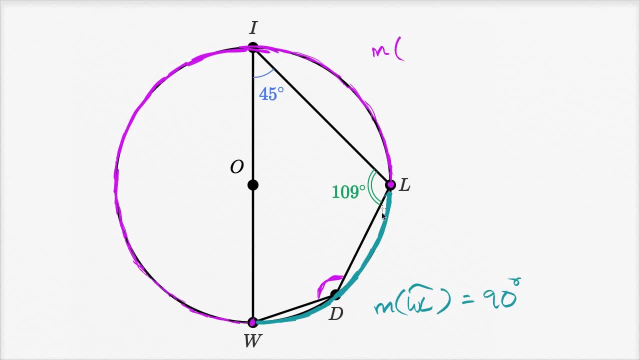 So, the measure, the measure of arc, let's see, and this is going to be, this is going to be a major arc right over here, This is so LIW, the measure of arc, LIW plus the measure of arc WL. 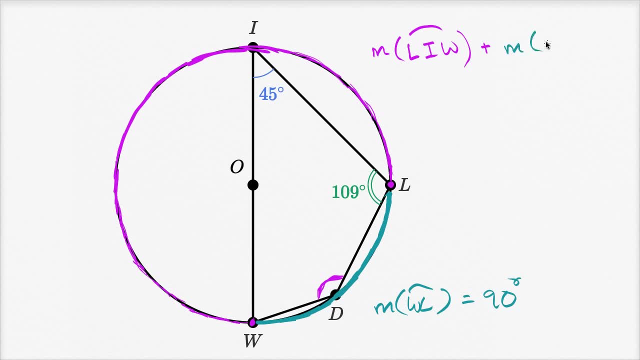 plus the measure of arc WL, plus this right over here, that's going to be equal to 360 degrees. This is going to be equal to. this is going to be equal to 360 degrees. Now we already know that this is 90 degrees. 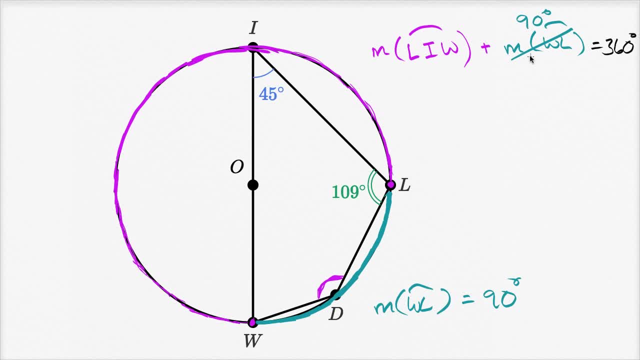 We already know WL is 90 degrees. So if you subtract 90 degrees from both sides you get that the measure of this large arc right over here, measure of arc LIW, is going to be equal to 270 degrees. I just took 300,. 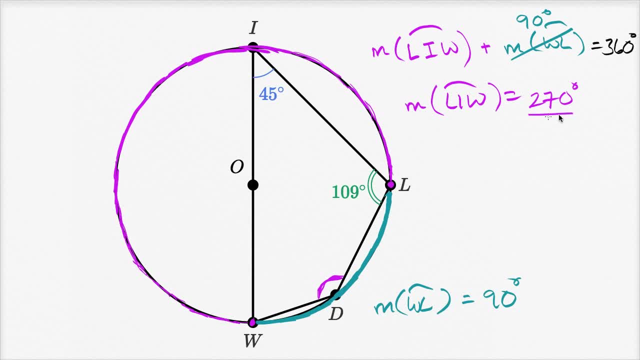 I went all the way around the circle, I subtracted out this 90 degrees and I'm left with 270 degrees. So let me write that down. This is the measure of this. arc in purple is 270 degrees And now we can figure out the measure of angle D. 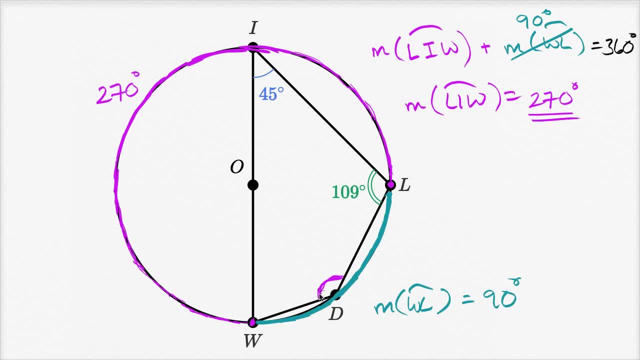 It's an inscribed angle that intercepts that arc, so it's going to have half the measure, The angle's going to have half the measure. So half of 270 is 135 degrees And we're done. And you might notice something interesting.